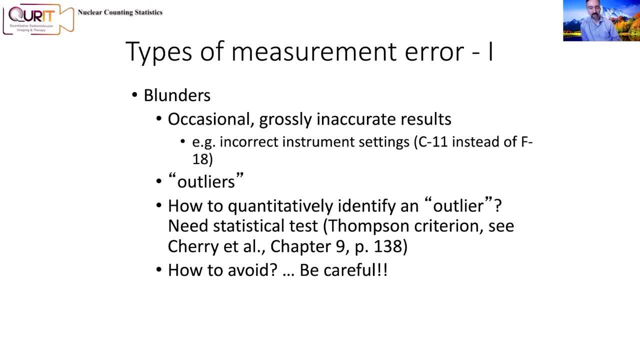 it away. You will go back and try to correct it. I remember years ago- this is like maybe 20 years ago- we had an invited speaker here at the physics department at UBC And just before he was here to arrive to give a talk, he won the Nobel Prize And I think he was from Stanford And in fact 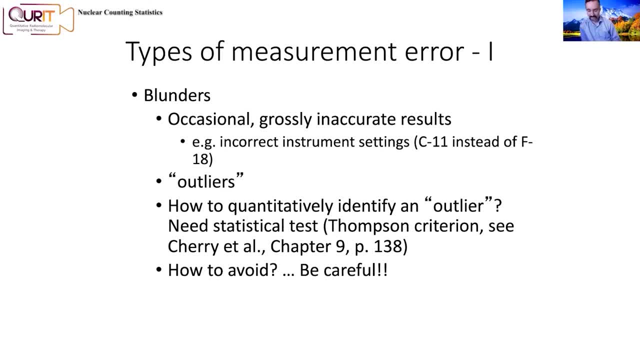 once I actually saw him in Stanford, just by total accident, And he said: well, you know I'm going to do this, And he ended up honoring the invitation. He showed up And he gave this lecture And the room was packed with people. This is so exciting. This guy just won the Nobel Prize in physics. 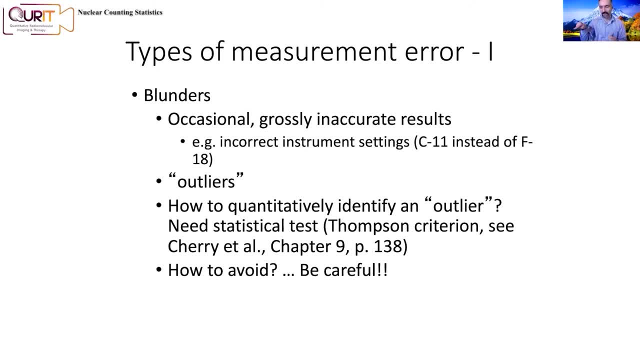 We were sitting watching him And I remember he showed this diagram And he said: this is why I won the Nobel Prize. And the diagram had, like it was supposed to give you, a nice linear fit. But he noticed that after a certain point he couldn't fit the data with the line And he had 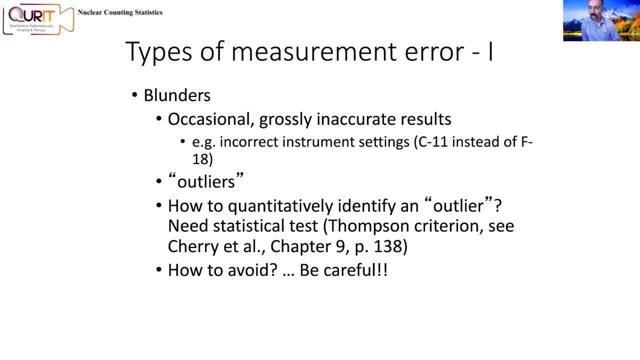 to change the slope a little bit And he could have called it an outlier and told me to do this And he totally ignored that point. But he ended up actually paying attention to this phenomenon. He ended up discovering this whole phenomenon. I think it was helium related or 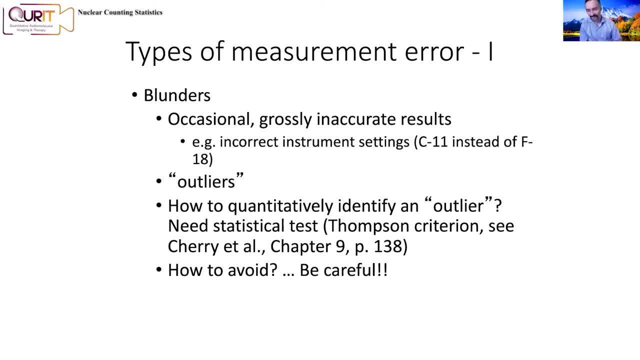 whatever it was, And he won the Nobel Prize. So I'm saying that you can't just get rid of outliers. Outliers often allow us to have major discoveries, Or sometimes they allow us to have major discoveries You have to understand. So often when we have outliers, we go back to the data And we 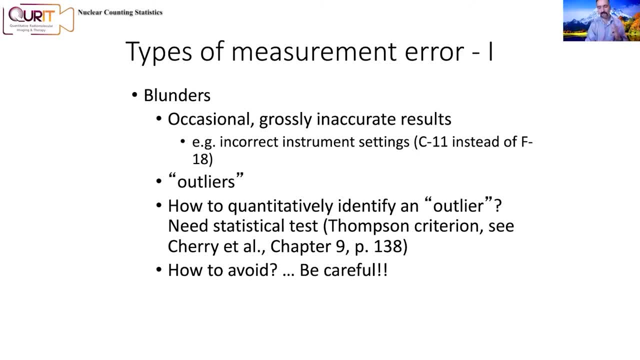 realize, oh, somebody did this wrong. So we redo the calculation And then we get the data to work better. So how to really avoid the outliers and then we get the data to work better. So how to really avoid the outliers and then we get the data to work better. So how to really avoid the outliers. 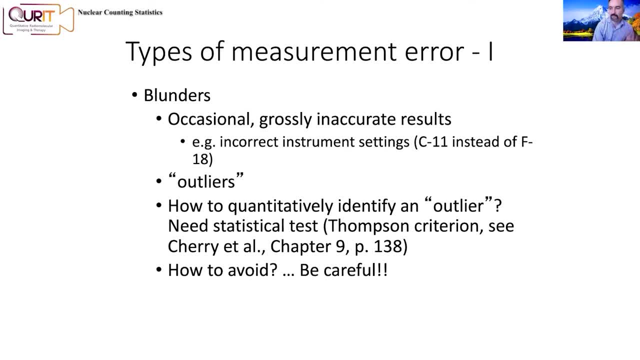 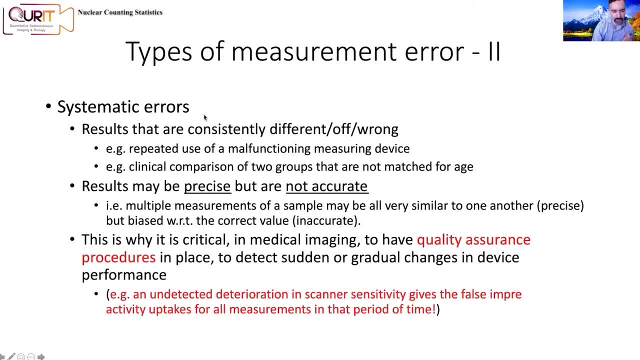 And once these are been avoided, you just have to be careful, But it will happen And you just have to go back and be systematic about it. But a far more common measurement error is systematic errors, And so these are things that are consistently different, or off or wrong. So repeat: 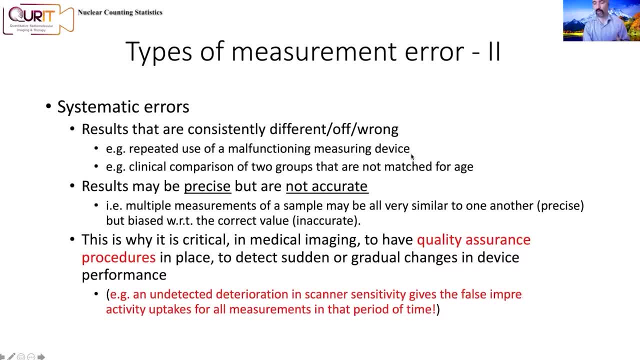 the use of a malfunctioning measuring device. If you have not done proper quality check- And we will have lectures in the future talking about quality check or quality assurance- If you don't do proper quality check, you may have a PET scanner or a spectrometer. 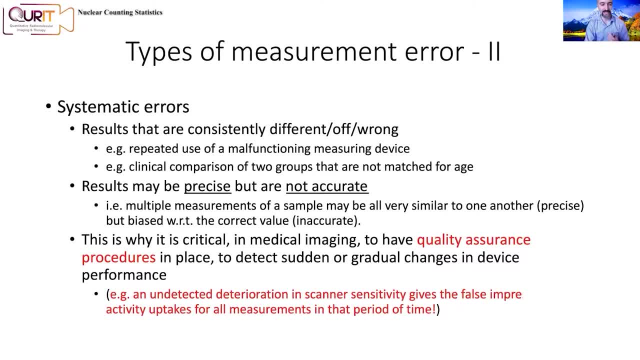 or a gamma camera that is malfunctioning and you're not realizing it. So it's consistently giving you wrong answers. And if you're comparing two groups that are not matched for age, for example, So results may be precise but are not accurate. okay. 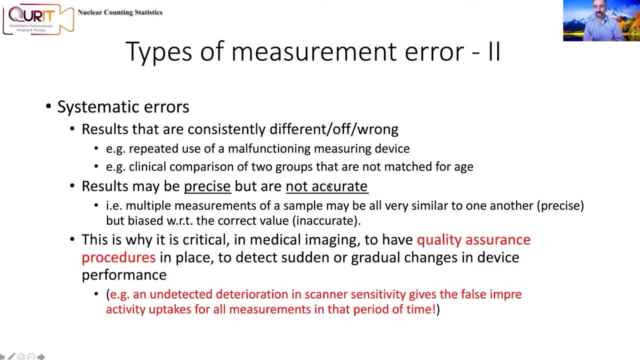 So this is a difference between precision and accuracy? I remember, just to give you another story, when I was defending my PhD thesis, I was kind of stressed out and people were asking me questions. Somebody asked me: what is the difference between precision and accuracy? 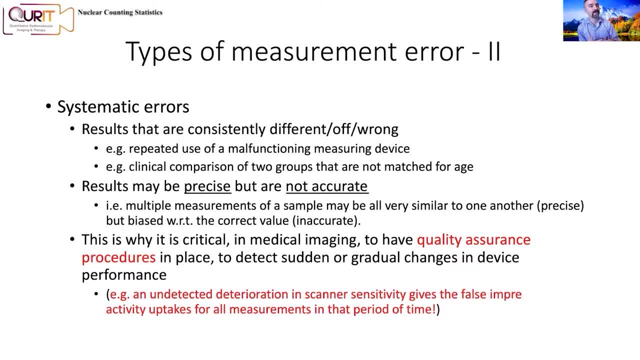 And I've said this to many people- I kind of I was stressed and I was like, oh, I just sort of guessed it because I was under pressure and I got it right. But this has always stuck with me. We should know the difference. 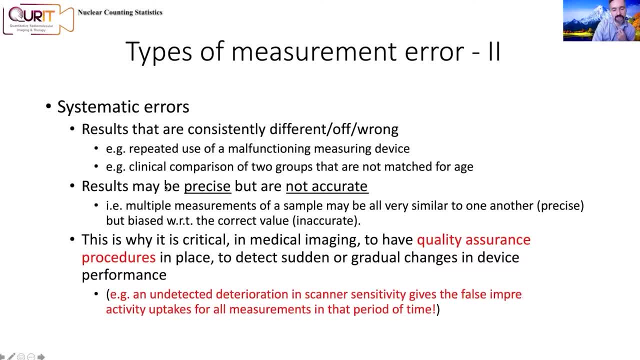 between precision and accuracy. So here we're dealing with something that may give you the exact same answer over and, over and over again, but this is the wrong answer, So you could tell someone you are precisely wrong, Right? So it's a systematic error. 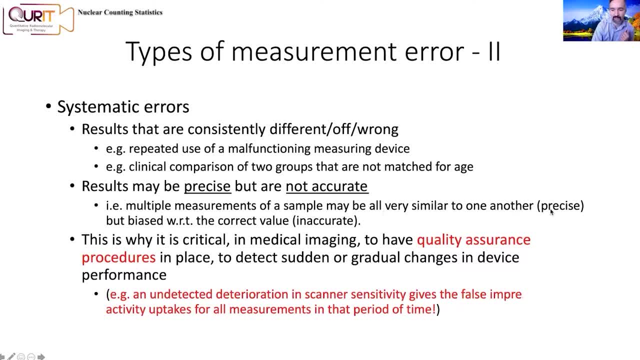 So multiple measurements of a sample may be all very similar to one another's as precision, but biased. Okay, so bias measures that, whereas noise measures the precision aspects: Bias versus noise. This is why it's critical to have quality assurance. So I talked about that. 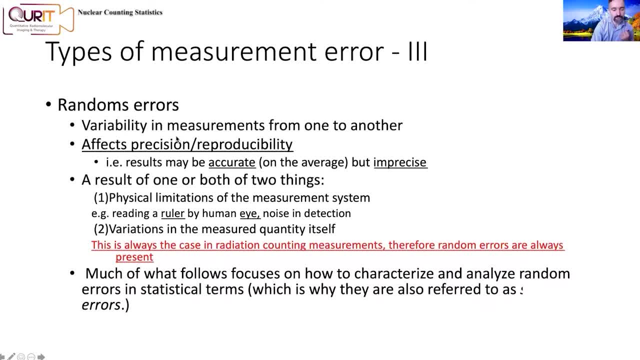 Okay, So random errors. and I remember how I said, in our field, radioactivity is inherently random. Okay, So we have an inherent randomness to radioactivity. On top of that, you know, device measurements also have their own randomness. If you read something on a ruler. 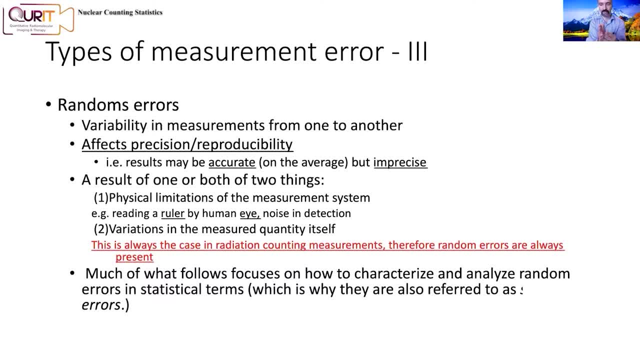 depending on the time of the day you're reading, or you know when you keep repeating it. you may read the number to be. you know a distance to be. you know 23.1 millimeters. The next day, you may read the exact same thing. 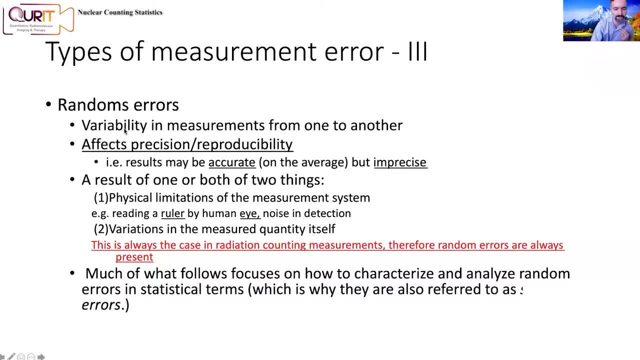 23.2 millimeters. These are random errors that you may actually have from day to day, Okay, Okay, So a result of two things: either physical limitations of the measurement system, So reading a ruler by human eye, So there's noise in our detection. 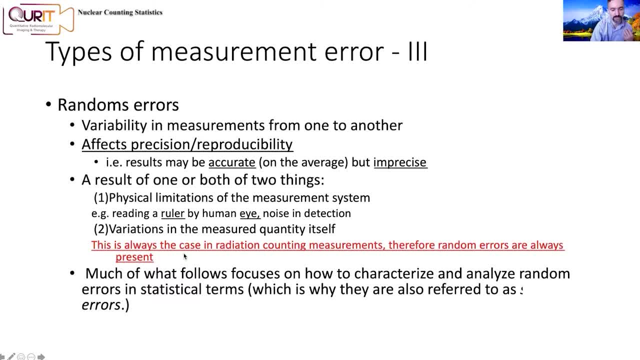 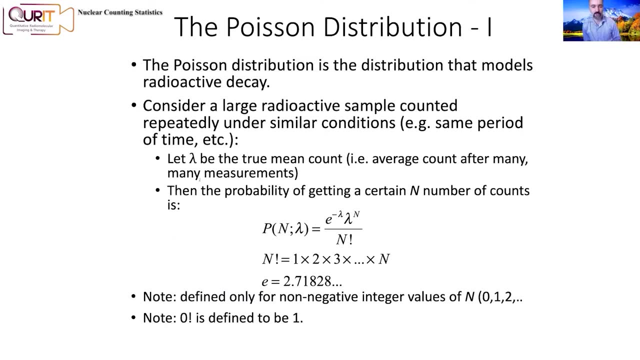 And variation in the measurement measured quantity itself. So this is always the case in in radiation counting measurements. Okay, Much of what follows focuses on how to characterize and analyze random error in statistical terms or statistical error. So Poisson distribution is a very, very important distribution. 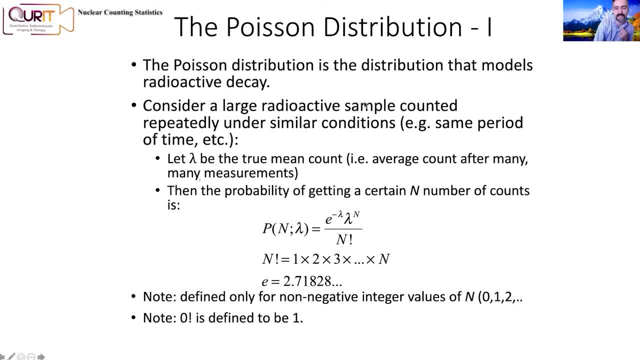 If you have a large radioactive sample, counter-repeatedly you're going to have Poisson distribution. In fact you can derive the Poisson distribution. Assume you have many, many, many nuclei and only a very, very small fraction of them decay. 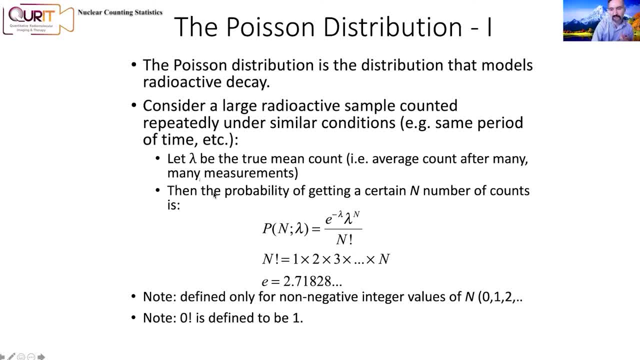 And that gives you the Poisson distribution And we won't derive it here. I think some of you might have seen it in undergraduate studies how this is the Poisson distribution formula itself is derived by that assumption. But the point is we have Poisson, the nature. 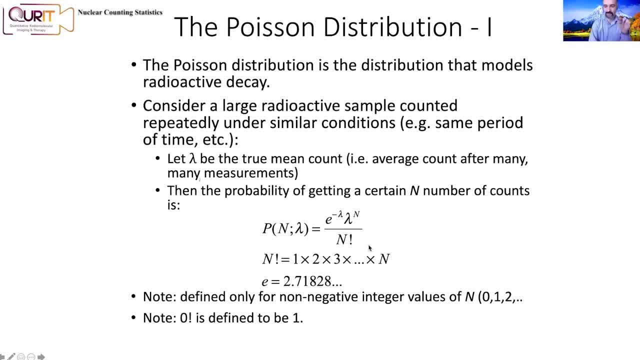 of radioactivity gives us Poisson. So if you have a detector, you have a sample of radioactivity. you have a detector here. in one moment it may measure 10 counts in another. Let's say you're measuring over one minute. first one minute. 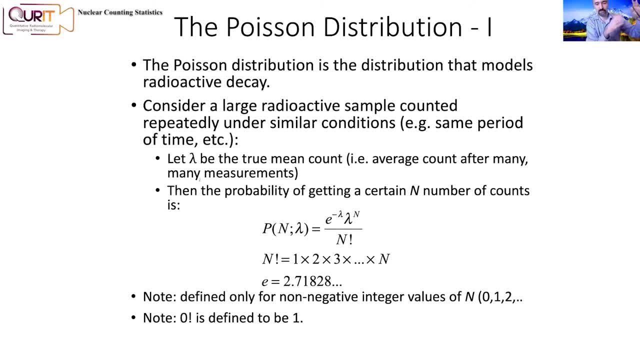 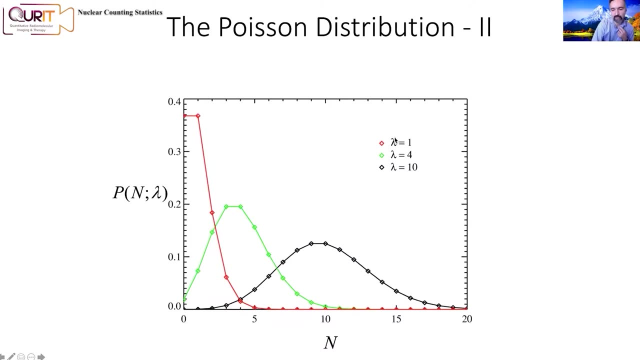 10 counts, another one minute, another day. nine counts, eight counts, 12 counts, 13 counts, that noise, that distribution of counts is given by a Poisson distribution which is given by this formula, And so you can sort of see if the true 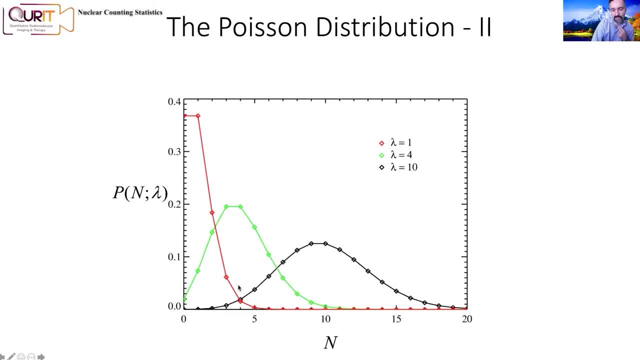 the mean is around one, the Poisson sort of spreads around. It's totally asymmetric because you cannot have negative counts obviously. So you're going to have a high chance of getting zero counts, one count and then less and less chance of getting two, three, four, et cetera. 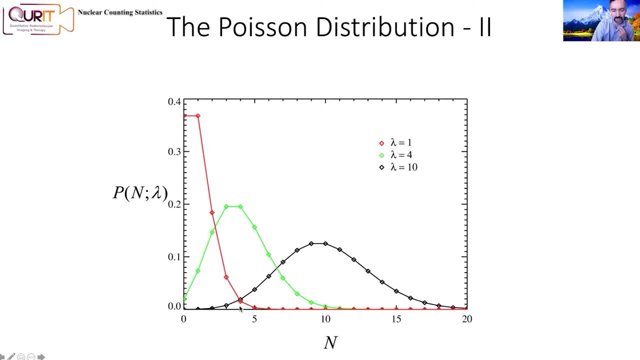 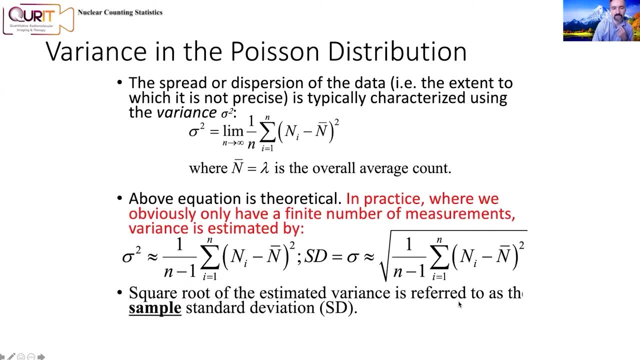 But if you have a land of four on average, if it's four- you're going to have a distribution like this, And as land becomes larger and larger, the Poisson distribution starts to look like a Gaussian distribution. Um, so variance is of course given by this formula. 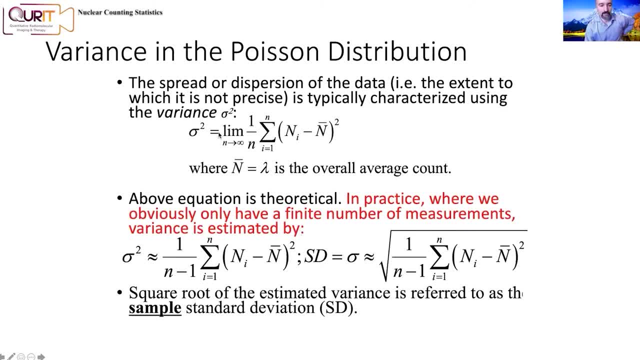 You all know this: The equations for uh, for uh, standard deviation and for variance, or variance, standard deviation is just the square root of variance. So this is the equation for variance. When you have an infinite number of uh, you know samples, uh, of course. 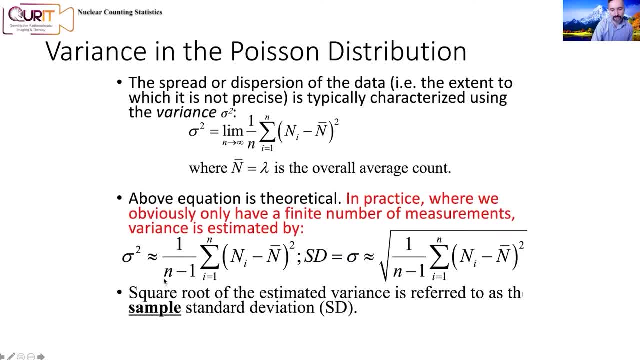 in reality, we do not have an infinite number of measurements. So often people, instead of saying one over N, they say one over N minus one. There is there is actually some good reasons why this is N minus one, Um some people actually. 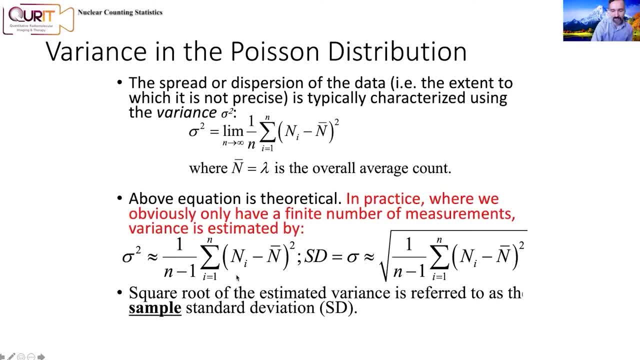 Disagree with this, but I won't go through that. but let's just use this equation for standard deviation. So so in this case we've got sample standard deviation. So sample standard deviation, uh, is an estimate of the true standard deviation. 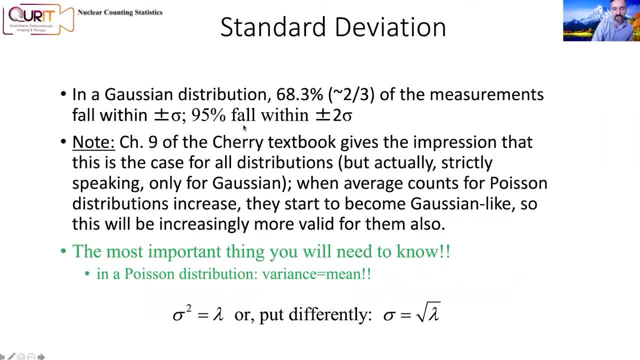 Um, anyhow. so you do that and in a Gaussian distribution, about two thirds of your measurements fall within one standard deviation and 95% fall within two standard deviations. in the cherry text, You may get the impression by reading it that this is true for all distributions. 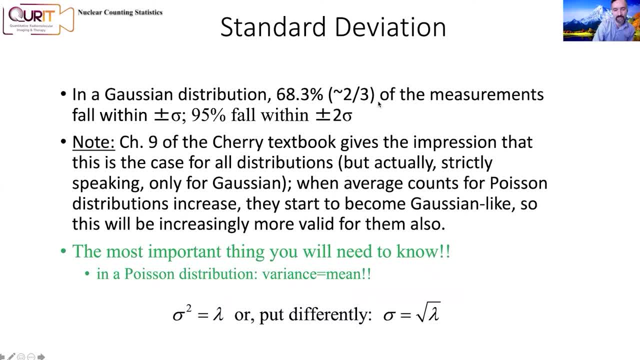 but it definitely is not true for all distribution. This is true. This two thirds is for true for Gaussian and for Poisson. Therefore, it's also true if you have larger number of uh mean values. but the thing you really have to remember for Poisson distribution, which is different, 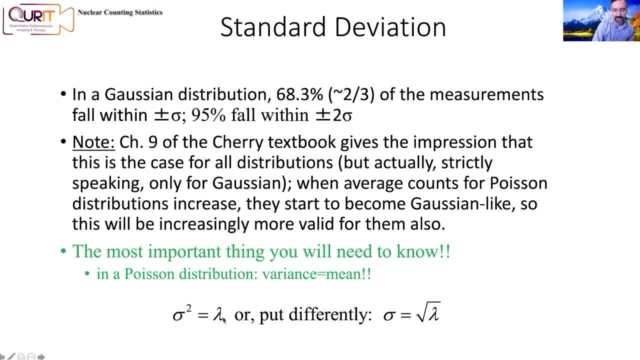 than Gaussian is that in Poisson distribution, the variance and the mean are intrinsically tied to each other. It's not. you don't have freedom, You cannot have a mean and a freedom of choosing your standard deviation, Unlike a Gaussian. the variance is equal to the mean or the standard deviation is. 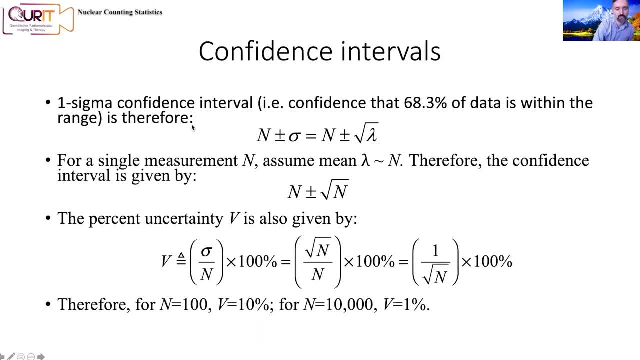 equal to the square root of the mean. So if that's the case, and assuming sufficiently large mean numbers so that we can use this, two thirds or 68% of the data, essentially this means that um about two thirds of your data falls. 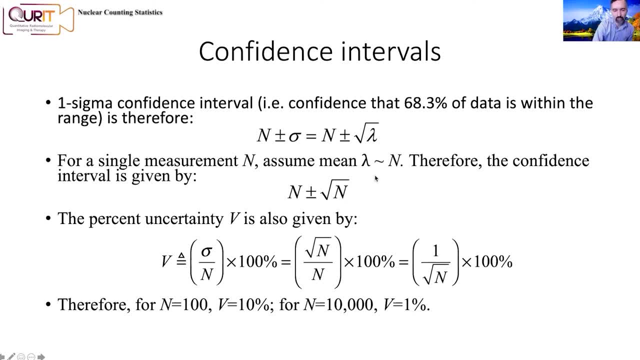 Within um, the number of counts plus or minus the square root of that Um. now, if you have a single measurement, um, well, you don't know what the true mean is, So you sort of S assume that the mean is equal to that single measurement. 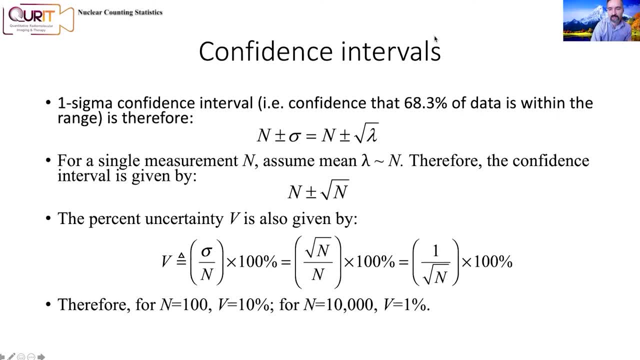 So we write this rule like that: Let's see, are we having questions here? Um, okay, So so we will. we will, uh, get back to that. Uh, yeah, let me. let me go through those three measurements. 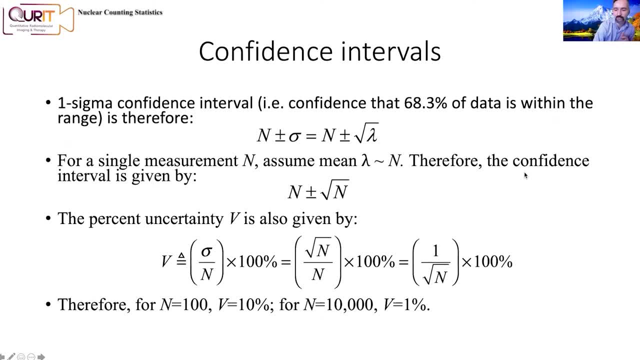 Feel free to ask questions. I mean, there's no problem in asking any questions you like. So we will answer some, we won't answer some, It's totally fine. So please let everybody ask questions as they wish. Do not stop yourself from asking questions. 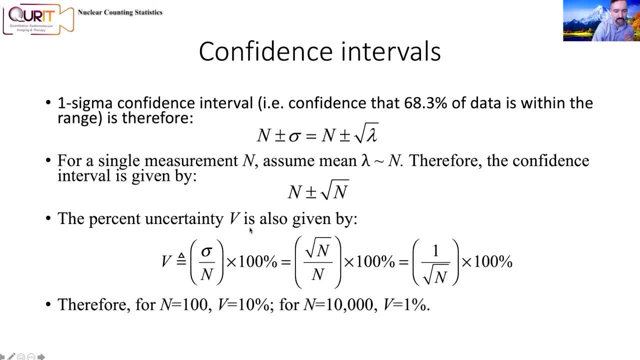 Totally fine to ask any question that comes to your mind. Um, so the percent? uh, uncertainty- is given by this formula, And therefore we've got square root of N divided by N. So it's this formula. So we've got a hundred counts measured by. 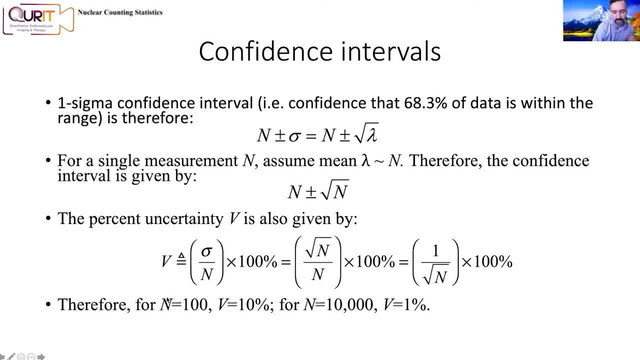 Well, in Poisson distribution the standard deviation is a square root of that. So it's 10 divided by a hundred, So it's 10%, you've got 10,000, then it's a hundred. square of that is a hundred. 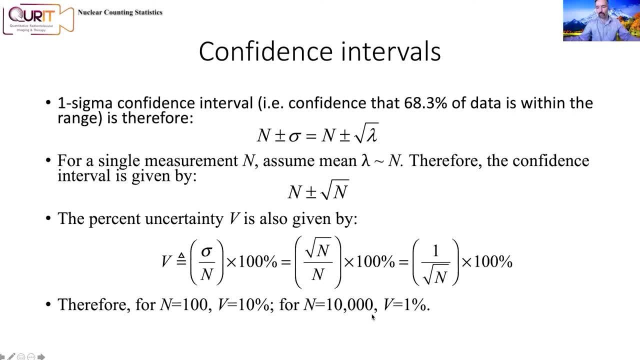 a hundred divided by 10,000 is 1%. So obviously, as you can see, if you count for longer, so you collect more counts. you're more certain, there's less variance. So just remember this formula: the square root of N is a standard deviation. 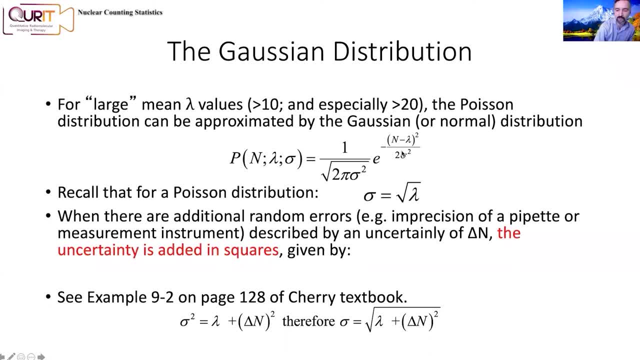 Um, whereas in a Gaussian distribution that is not true. in a Gaussian distribution, Again, the mean can be different. Then this totally decoupled from the standard deviation. but in a Poisson distribution that's not the case. These two are inherently linked to each other. 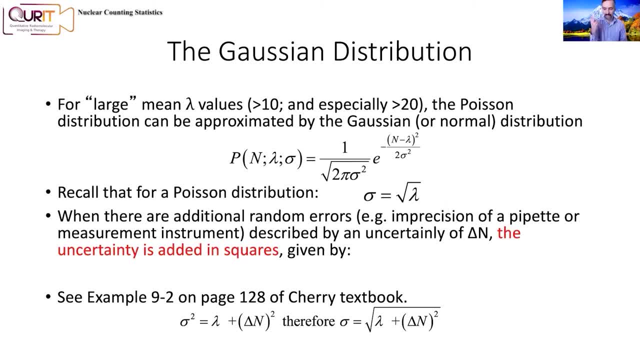 So, in a sense, you only have one degree of freedom, unlike a Gaussian which has two degrees of freedom. Um, so here's a, here's an examples on what happens when you have additional random errors, Like: uh, for example, you have a error in the measurement instrument that you add to it. 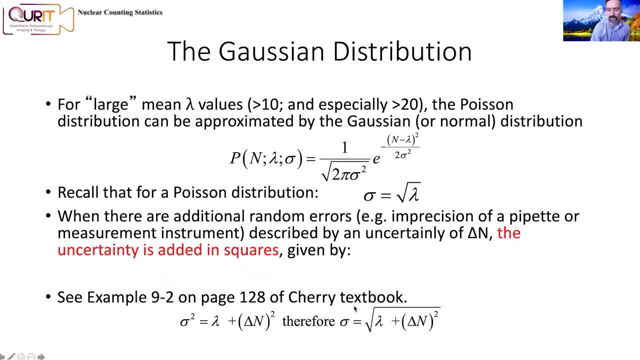 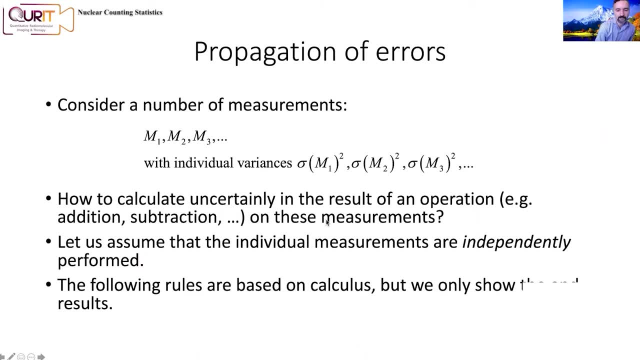 You can refer to this cherry textbook if you have it. if you don't have it, don't really Worry about it at all. We're not going to ask you questions if, if we're not providing you the material, Um unless the question is directly using this equation that you're being provided now. 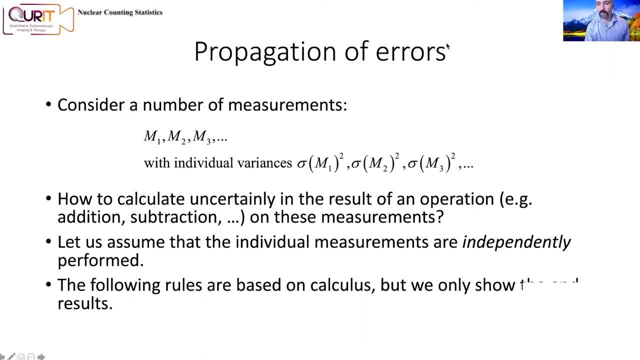 So how do you propagate errors? Um, how do you propagate errors? Um, yeah, so so we're asking a question. Uh, thank you, Yvonne. Fantastic question: Why is Lambda equal To the mean? um, yeah, so I think there's. this lander is not necessarily the same lander as we had before. 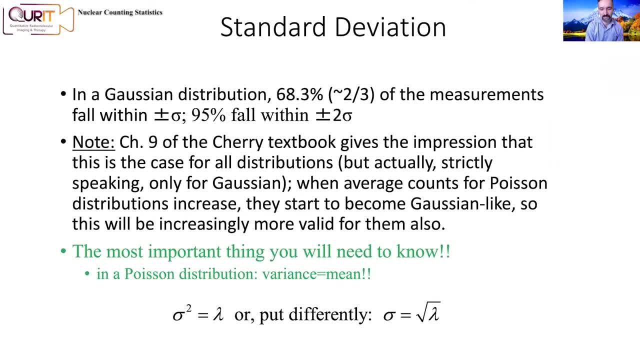 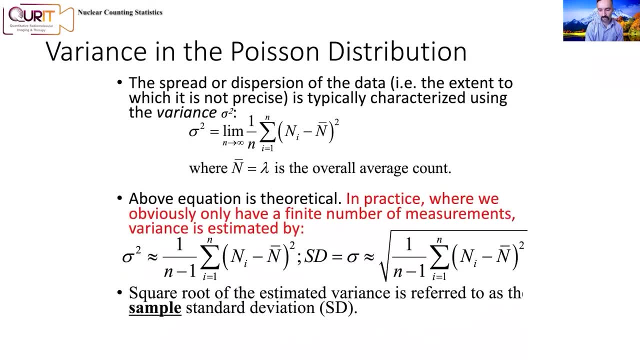 So I want to be very clear. Uh, let me go back to the notes. Yeah, I think that might create some confusion here. The lander that we use in the Poisson formula- this is not the same as the lander we were talking about as the long term. 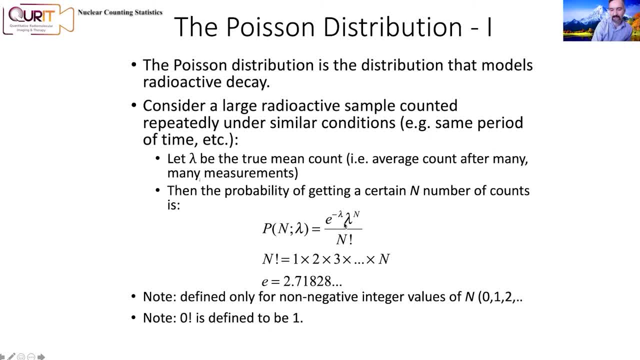 It's not the same as the law of decay before, so that's just a similar land. It looks like the similar lander, but it's not the same lander. So here's by Lambda We simply mean. that mean count is the actual average number of uh radioactive decays. 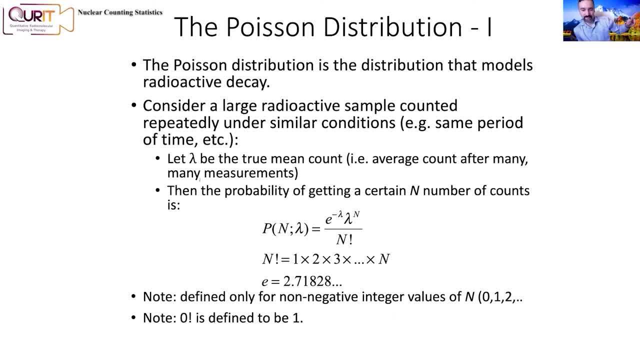 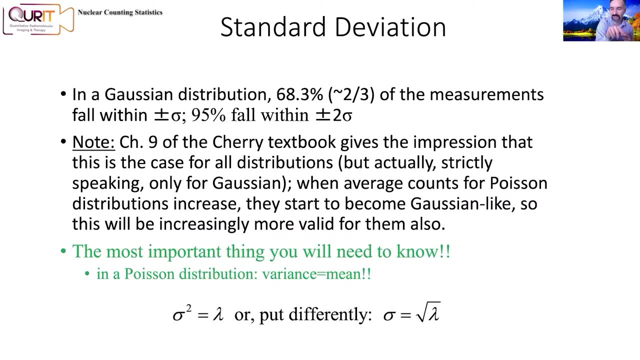 Whereas previously Lambda was the decay rate compared to the total number of counts. So it's not the same. Good question. So thank you. So I hope that answers well. Yeah, This lander is different than that lander where we had, you know, the exponential law e to the power of minus Lambda t. 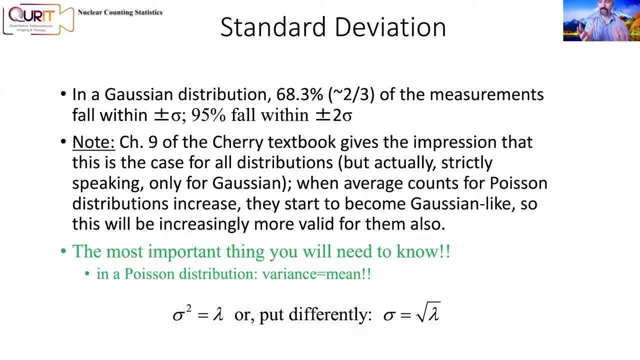 This lander is not that this lander is. let's say you have a one, you're measuring something in one minute. What is the true number of average counts you're going to measure in one minute in this sample? That's Lambda. 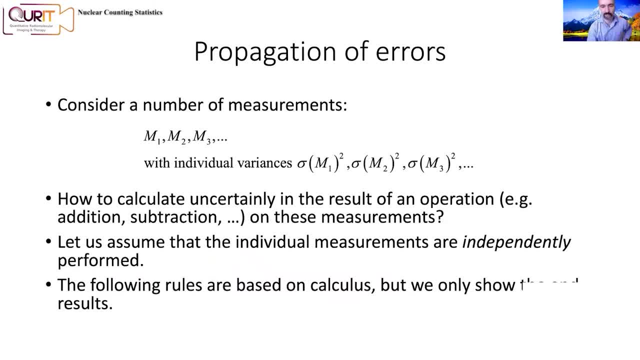 Thank you, Great question And thanks for that, Helping me clarify that you want Um. so how do you propagate errors? You've got different Means, different landers, You want to do subtraction, addition, et cetera. How do we do it? 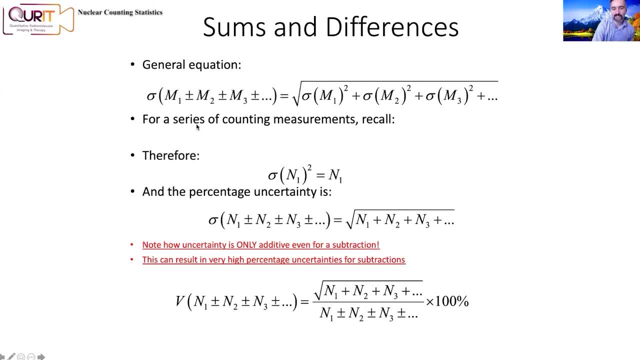 Well, this is a general formula, has nothing to do with radioactivity. This is just general formula. You guys should know, when you're adding uncertainties or subtracting uncertainties, the the error in them always adds. even if you're subtracting, the error ads in squares. this is a general formula. 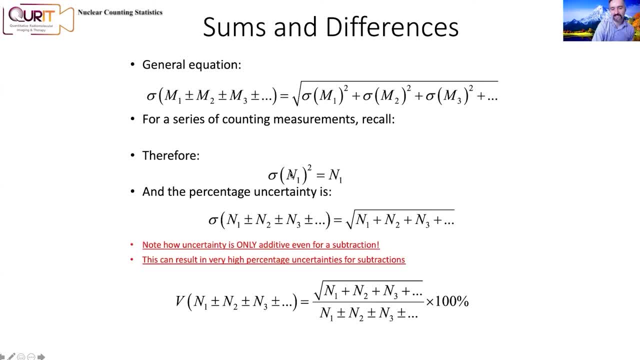 Now, of course you could. you know, you could do the math and say: Sigma squared is equal to N In the case of Poisson distribution. So you can substitute and get this. Frankly, I don't memorize these formulas in the cherry texts. 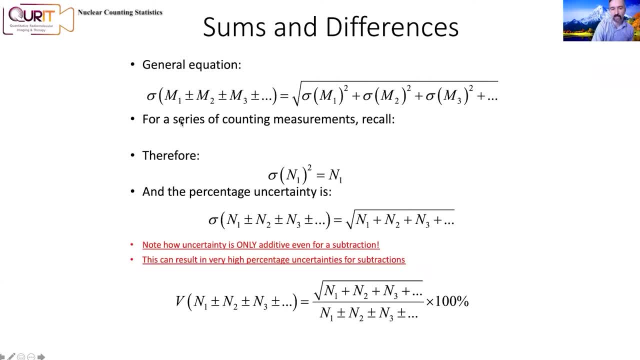 They have all these different formulas. I really don't memorize these at all. I only know this, And many of you already know this from undergraduate studies- that when you add or subtract uncertainties, the associated lander just adds in quadrature. and you just have to know this additional rule and you're set to go. 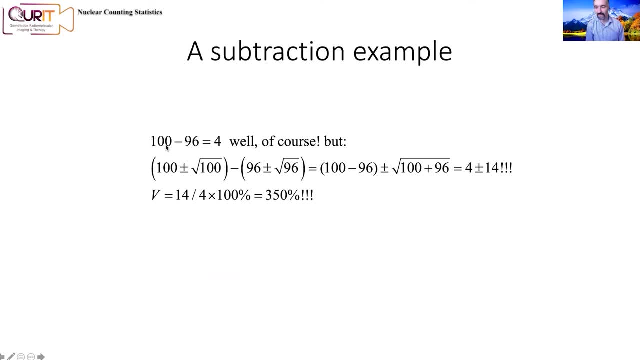 So, for example, what's a hundred minus 96.. That's a great, uh, you know great uh. what is it? Three question, or whatever? Of course we're not testing anybody doing this- but what is a hundred minus 96 in terms of noise propagation? 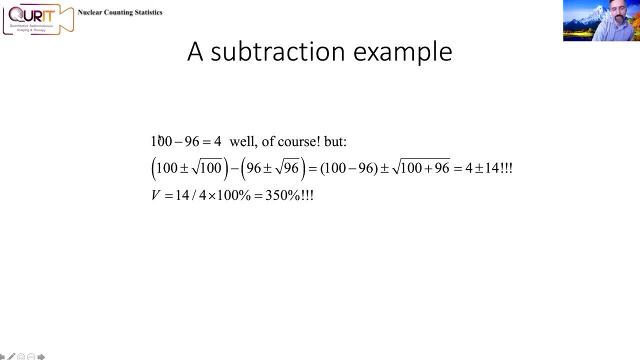 So so you've got, a hundred is plus or minus square of a hundred. So if you measure- if, for example, you measure a hundred counts and in some study and I measure 96 counts in other studies- somebody asks you: what is the difference between these two? 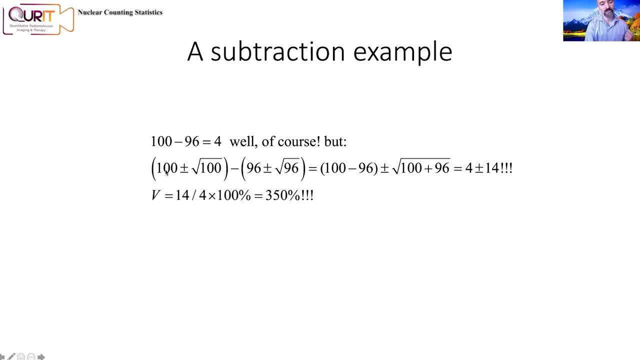 Well, obviously it's four, but four plus or minus, what? So? it's a hundred plus or minus square of a hundred, minus 96 plus or minus square of 96.. And these, as we said before, they add in quadrature. 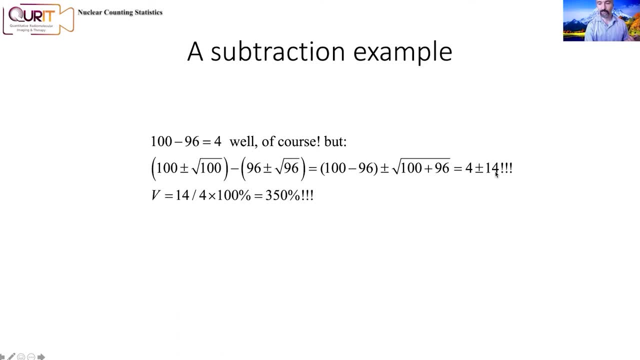 So you square this plus square of that, You take the square of that, you get 14.. So actually subtraction can give you very large errors. So we've got four plus or minus 14. That's like a 350% error. 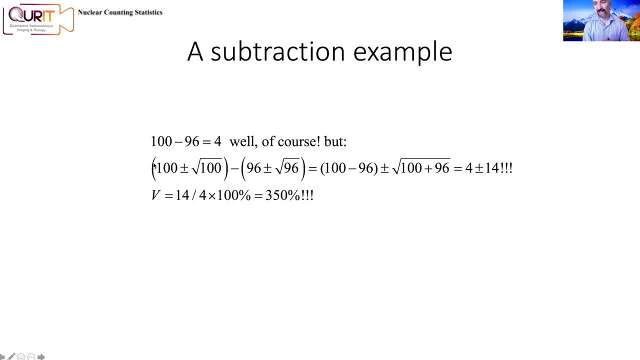 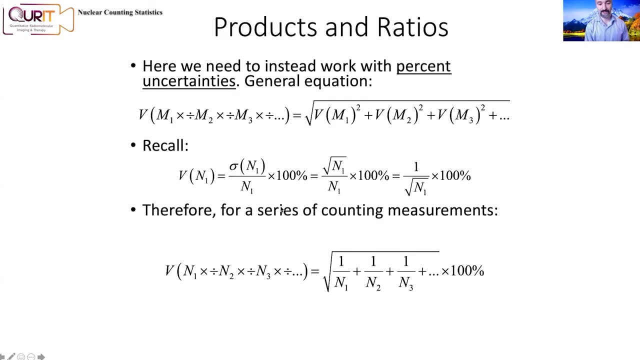 So we're very, very uncertain. If you measure a hundred counts and I measure 96 counts in a, in a counter the difference is four. but we're very uncertain about how true that is. Now for multiplication and division. Again, you've seen this in undergrad. 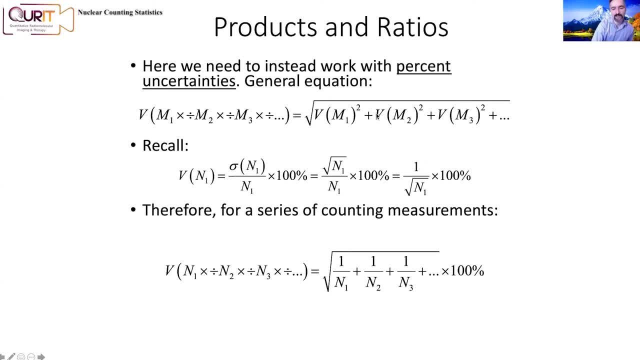 You've seen this in graduate studies. if you're multiplying or dividing again, you add only, but you add the percent uncertainties, not the absolute uncertainties. So first you have to convert your standard deviation to a percentage, Then you add them in quadratures. 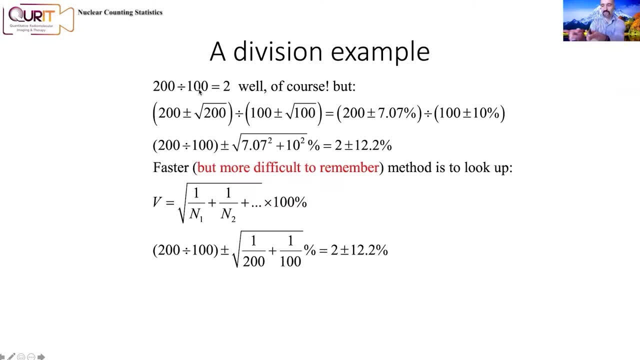 So again, let's ask you a question: What's 200 divided by a hundred? You measure 200 counts, I measure a hundred counts. Somebody asks you: what is the ratio between these two measurements? Well, of course it's two, but two plus or minus what? 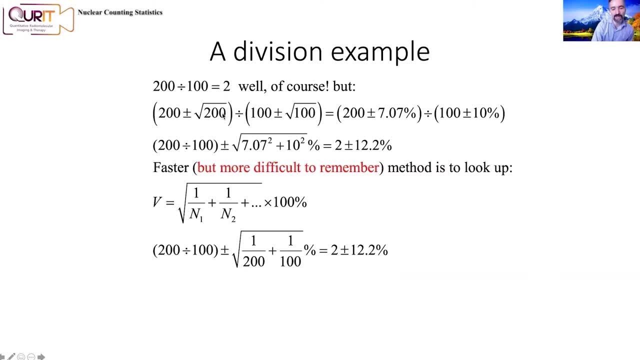 How certain am I that this ratio is two? Again, you go through the math. This is 200 plus or minus square root of 200, but you have to convert this now to a percentage. So 7% for this and 10% for that. 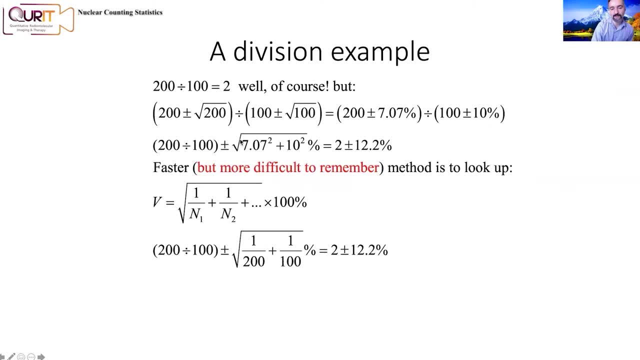 Then you add this 7% and 10% in quadrature like this and you get this number. So the ratio of these two numbers is two plus or minus 12%. Again, you could sort of put these equations in there. blah, blah, blah. 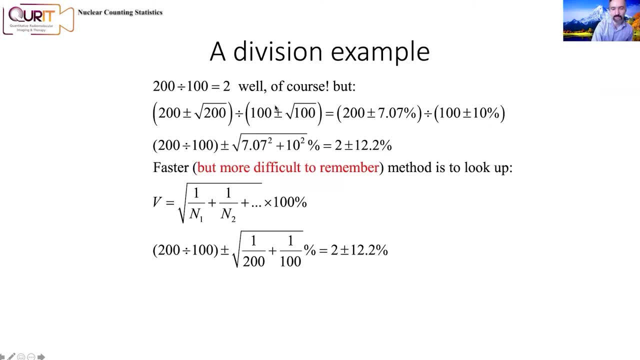 But I really don't memorize these at all, Even though there's some textbooks write them. I just memorize the general And then I just know that you just have to put the square root for the standard deviation. That's it. Now, if you're doing a constant multiplier, well, it's very simple. 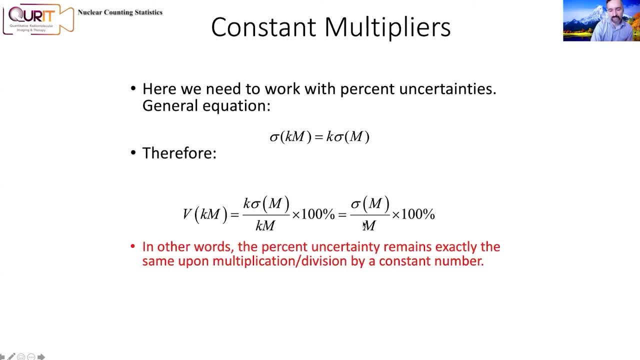 And you can easily prove this- The percent error remains the same. You can show it because the standard deviation simply multiplies. So if K is a constant multiplier, like a fixed number, like if there's zero uncertainty associated with K, Like, let's say, you just say: 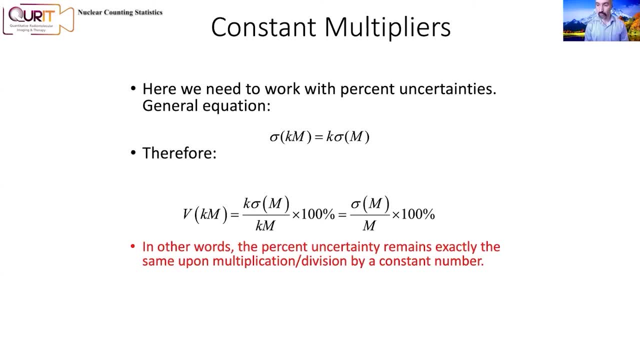 You gave me 200 counts. What's that? multiple by two? an exact two, not an uncertain to an exact. I just want you to multiply that by two. If you were counting, you know twice as much, what would you get? 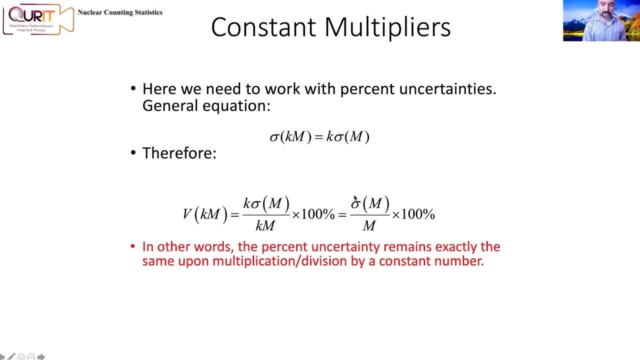 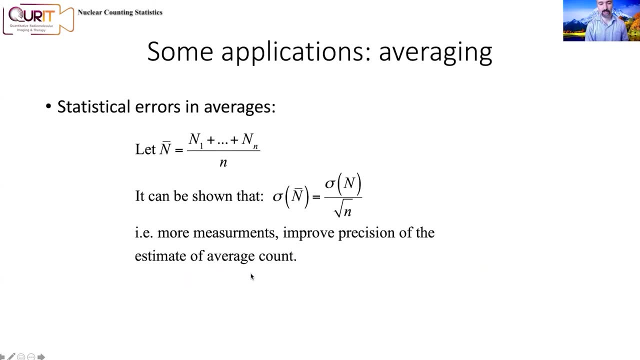 Well, it's twice as much in absolute standard deviation, but in percentage it's the same percent error. So therefore, the percent uncertainty remains exactly the same by multiplication or division by constant number And finally, if you're averaging. this is why averaging is such a good thing. 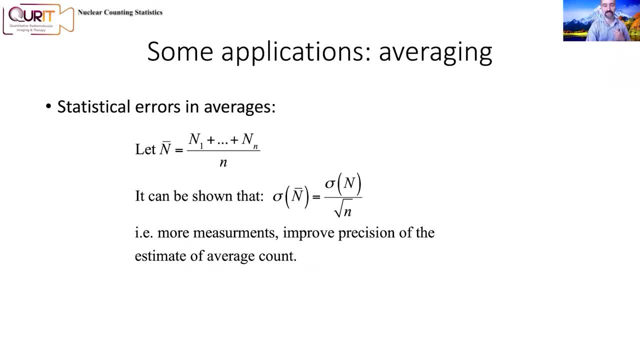 It's good for all of us- multiple of us- to be making Measurements and then averaging the results, because it turns out in general that the standard deviation of the mean is equal to the standard deviation of in one measurement divided by square root of the number of measurements that we're making. 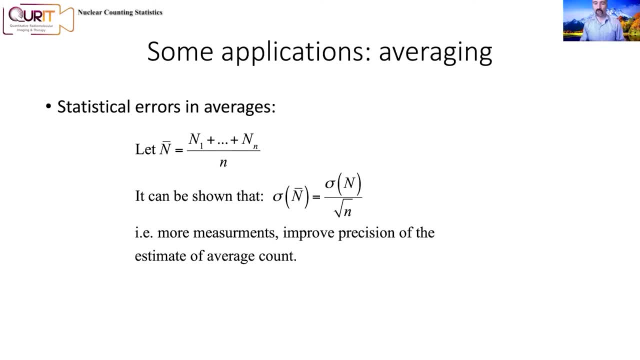 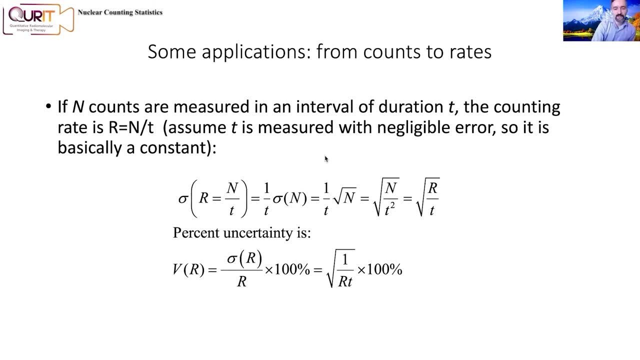 Number of samples that we are collecting. Let's say, 10 of us are going to the field and making you know measurements of something, And this is true in general. Now there are some formulas. Again, I don't memorize these formulas. 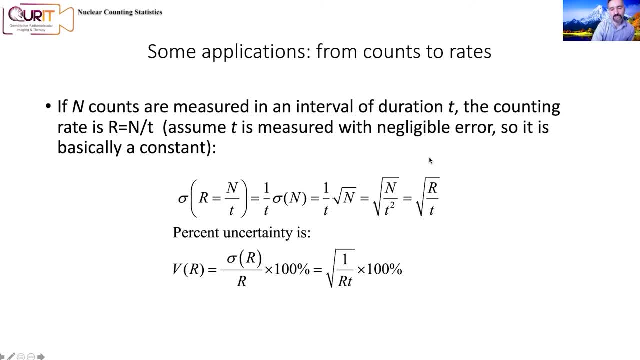 But you may want to Memorize. if you really were to memorize something, you may want to memorize this one, but I don't have it memorized in my own mind. So for count rates, you can actually show. a count rate is the number of samples you measure divided by time. 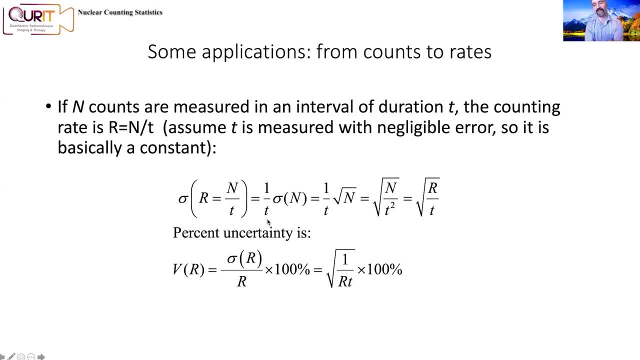 Remember time is a constant multiplier. Let's assume time you measure very, very, very accurately. Let's assume there's not much error associated with time. Then you have this formula, You put it in here and you can bring the T inside to get this. and over T is R. 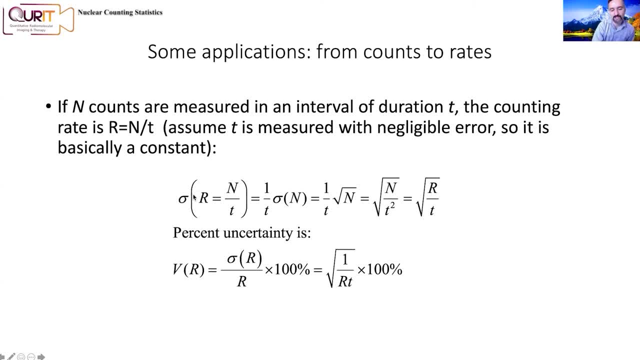 So you sort of get This equation. So the standard deviation of the rate- not the number of counts you measure, the rate of that you measure is given by this formula. Okay, And you can also calculate it for percent uncertainty. Again, frankly, I don't memorize this formula. 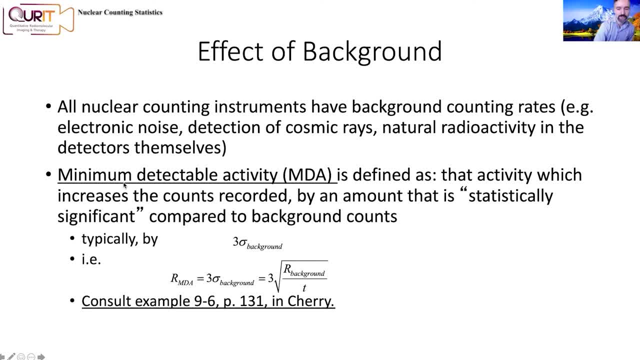 Now, effect of background radiation is important. There's this thing that we refer to. So you know, all nuclear counting instruments have some background counter rates. Um, And so this could be from electronic noise, detection of cosmic rays, natural radioactivity in the detectors themselves.